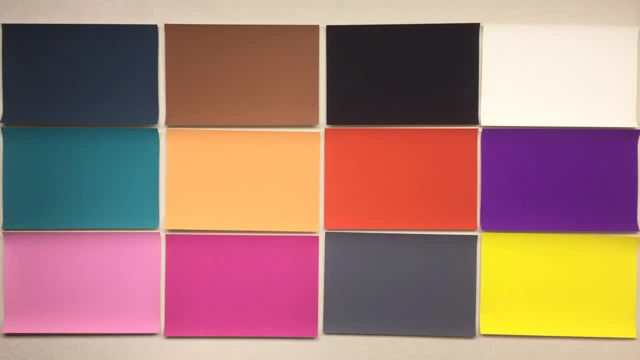 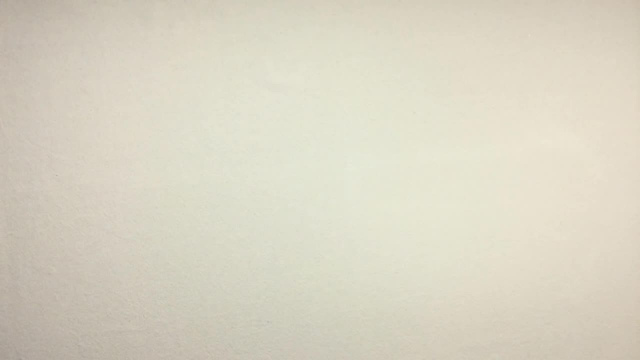 Colors are all around us. They seem simple, but they're actually the result of a complex interplay between physics and biology. But what are they and how do we see them? Color is the way our eyes and brains perceive light. Light is a wave and, like any type of 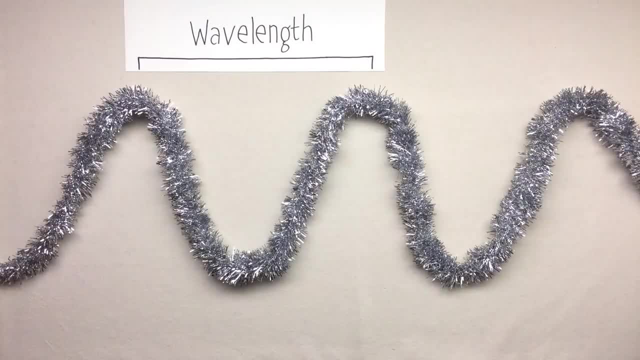 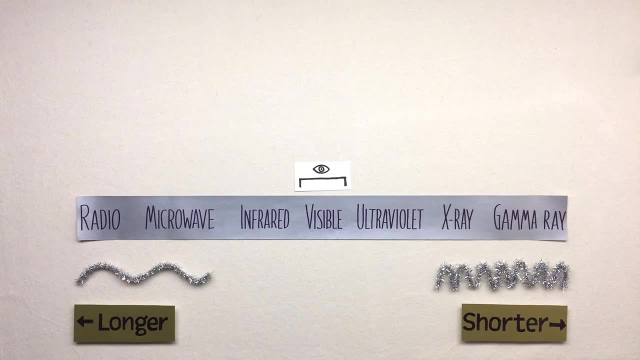 wave. every light wave has a particular wavelength, the length of each cycle of the wave. There are many different wavelengths of light, but we can only see light in this little range of wavelengths called visible light. Everything else is invisible to us. 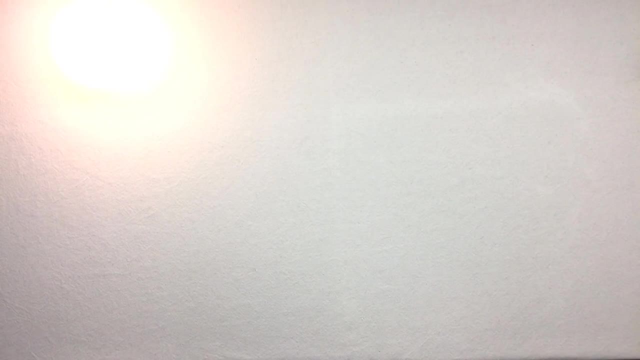 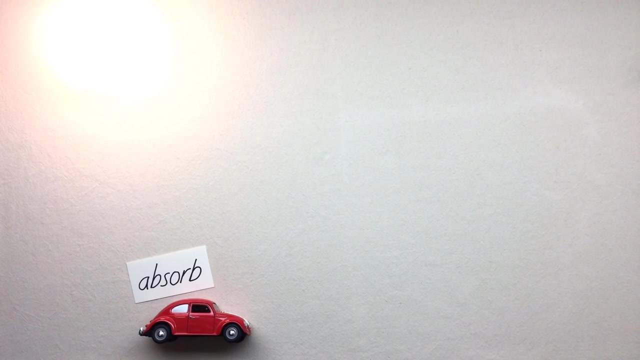 The sun is constantly emitting basically every wavelength of light. All those wavelengths are shining on this car. The car is made of a material that absorbs most wavelengths of visible light, But there's one wavelength in visible light that it reflects. Some of that reflected. 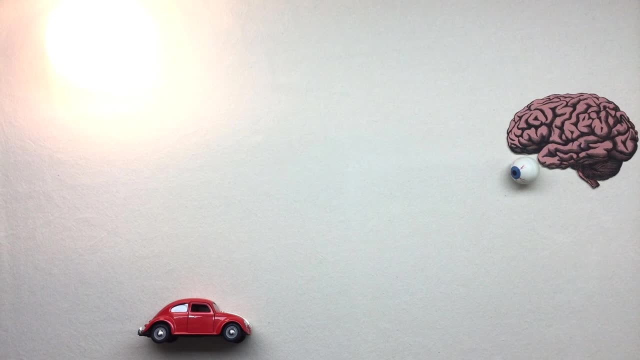 light goes into your eye. Your eye tells your brain about the light and your brain uses that information to make you have a particular perception of color. The color we see is based on the wavelength of the light. Red is just the breakfast table you spend with your peeps and your teachers while they're at your house and playingprü agrarian. Red is the building of your define of your brains. Red is the universal rokka lehmmls of your brain. Red is the light you spend about the life cycle of your life. Red is what make some people. Red is the 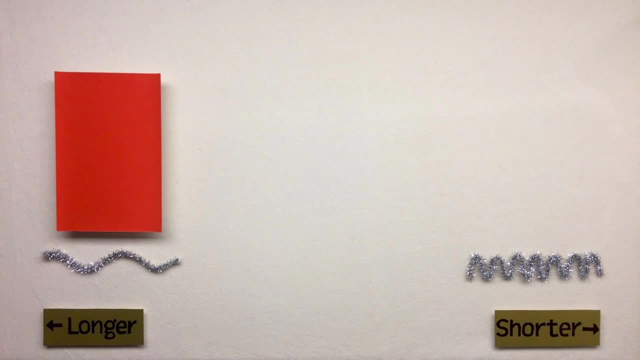 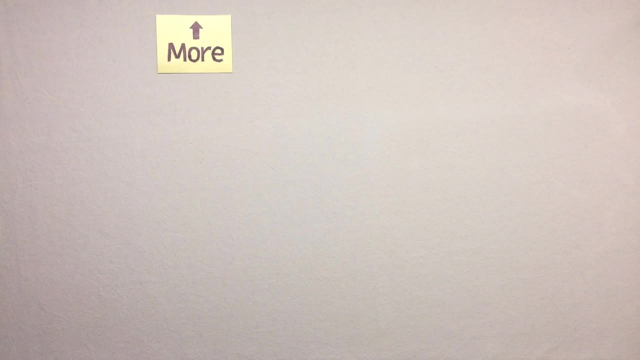 Red is how we see the longest wavelengths of visible light. then there is orange, yellow and so on. The wavelengths of visible light form the colors of the rainbow. Also, the more light there is, the brighter the color we see and the less light there. 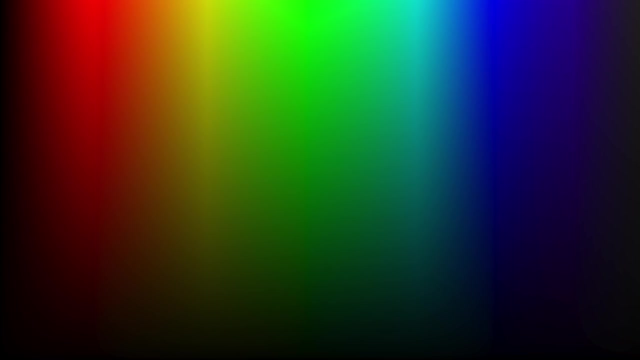 is the darker the color. This gives us multiple shades of all the rainbow colors. But there are more colors than these. What about white and pink and brown? Well, it turns out that most colors are more complicated than just one wavelength. 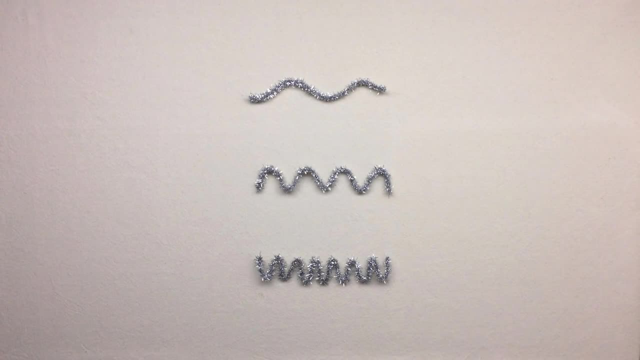 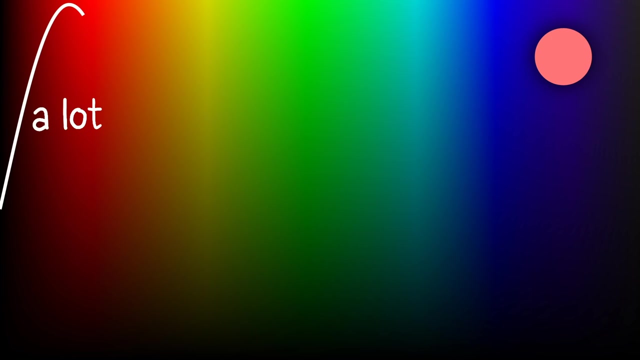 Most colors are a combination of multiple wavelengths. Specifically, we can say a color is a certain amount of each wavelength. For example, you see pink whenever a lot of red light plus a little bit of every other wavelength enters your eye. Brown is a medium amount of red light plus orange, plus yellow and none of any other. 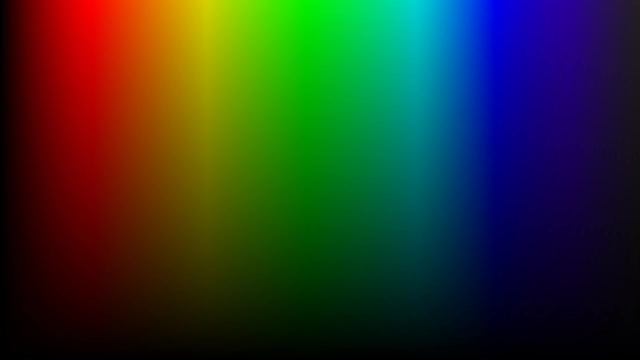 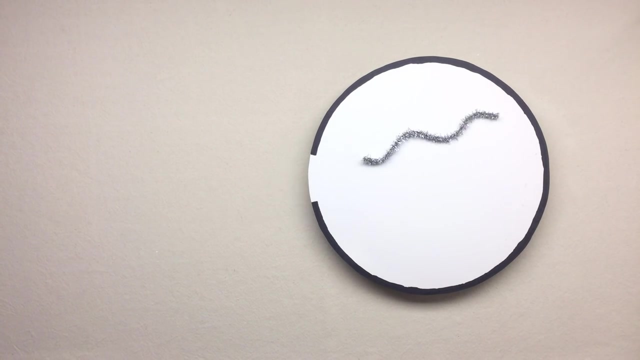 wavelength. White is simply a lot of every wavelength and black is none of any wavelength. But how do we see these colors? Well, when light enters your eye, it hits your retina, where there are light-sensitive rod cells and cone cells. 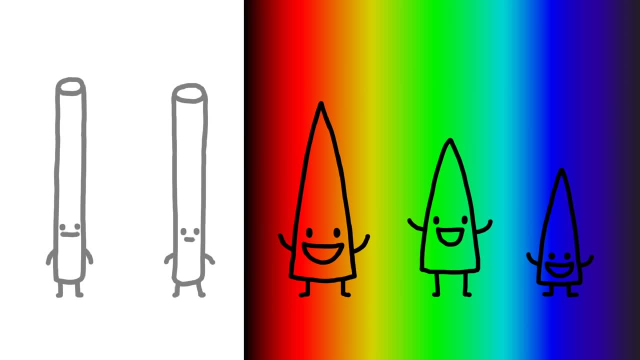 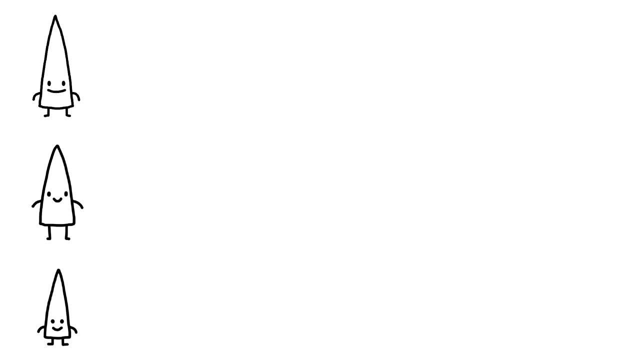 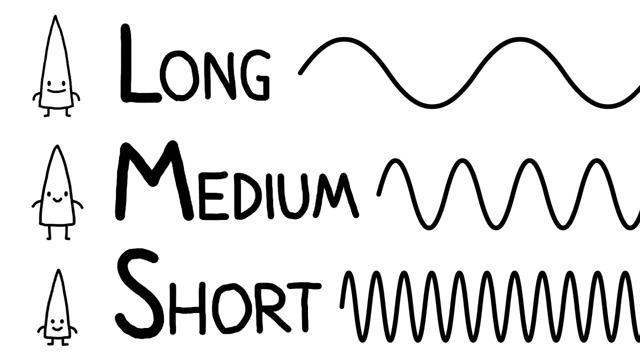 Only the cones are used for color vision, so we're just going to focus on them. There are three types of cones, and each type is sensitive to different wavelengths and different amounts. There are the L, M and S cones, most sensitive to long, medium and short wavelength light. 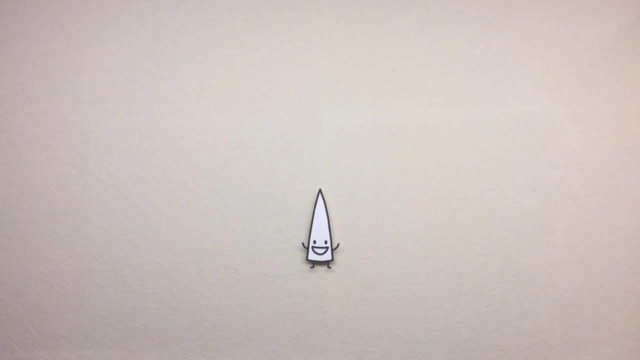 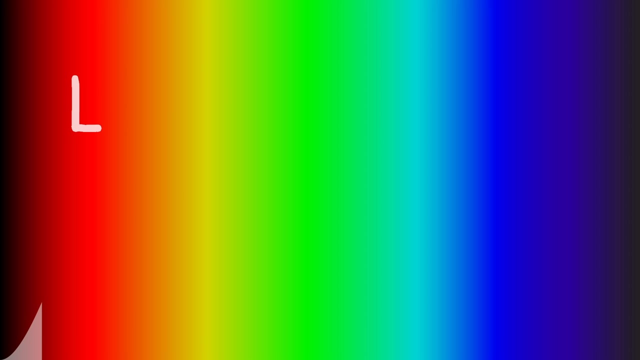 respectively. Each type of cone reacts a different amount to different wavelengths. Let's look at L cones first. They start getting sensitive around here with very low wavelength red light. Then, as the wavelength gets shorter and shorter, L cones get more sensitive. 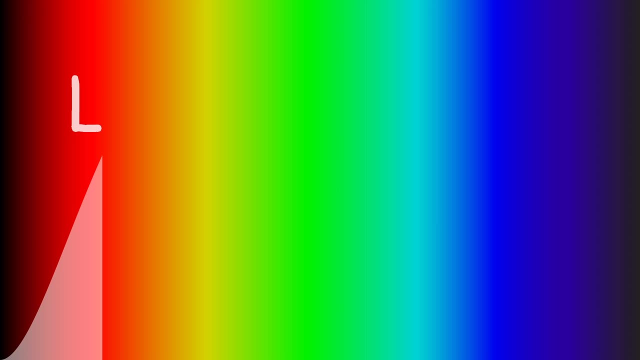 They start getting more sensitive around here with very low wavelength red light. Then, as the wavelength gets shorter and shorter, L Cones get more and more sensitive, eventually peaking in sensitivity at around yellow. Then the sensitivity drops back down again. L cones aren't sensitive to blue light. 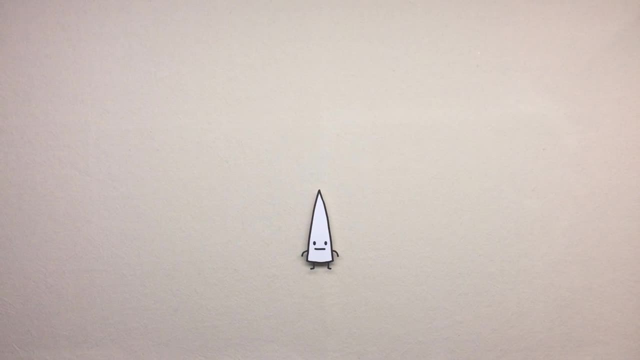 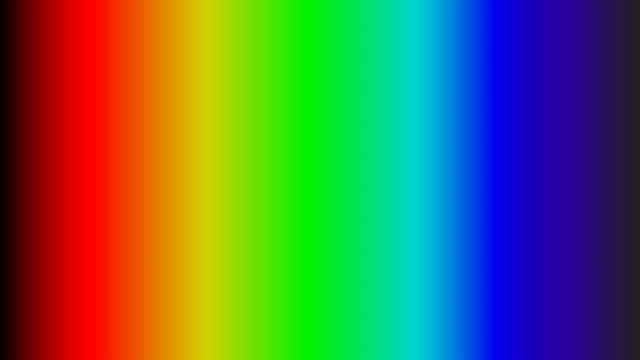 Finally, there's another little bump of sensitivity to violet. What all this means is that yellow light, for example, makes L cones react a lot, Green light makes them react a little bit, And blue light doesn't make them react at all. The sensitivity graphs for the other types of cones are just simple peak-shaped curves. 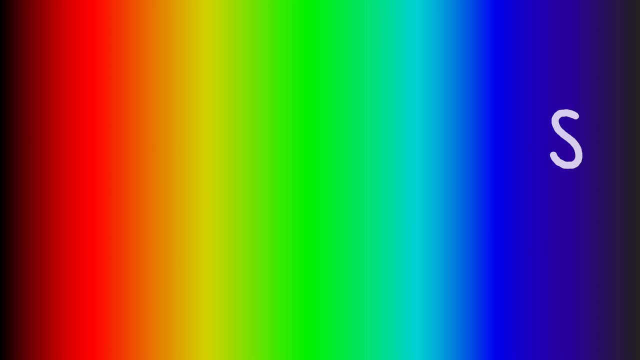 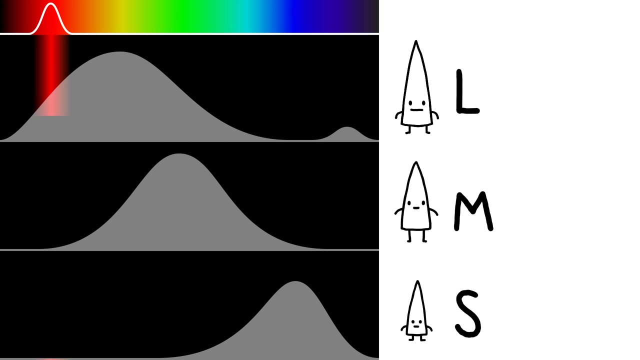 with the M cones most sensitive to blue light. The sensitivity graphs for the other types of cones are just simple peak-shaped curves to green light and the S cones to blue. Let's see how the cones react when pure red light comes into your eye. The L cones are moderately sensitive to this wavelength, so they sense a good amount of. 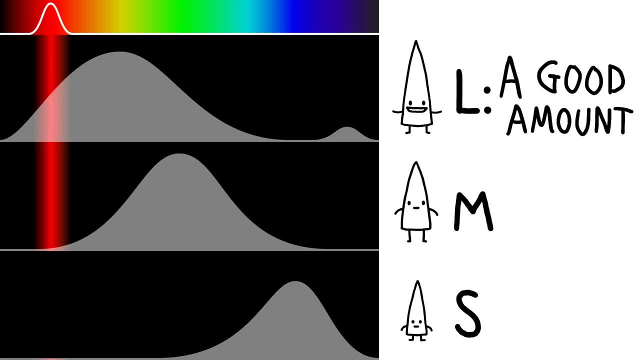 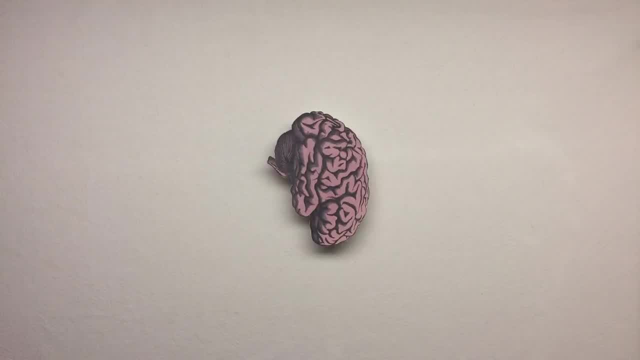 light. The M cones aren't sensitive to this wavelength, so they don't sense any light, and same for the S cones. Your brain takes in this information and, based on it, it makes you have the sensation called red. How about white? Well, since white is a lot of every wavelength, it. 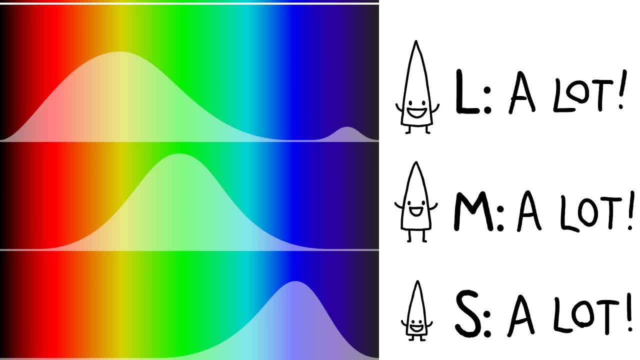 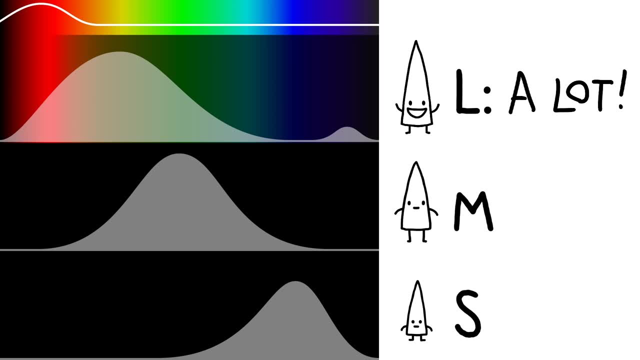 impacts all of your cones a lot. Based on these responses, your brain makes you see white And for pink, the L cone reacts a lot to the combination of the large amount of red light and a little bit of everything else, while that little bit of everything else makes the other. 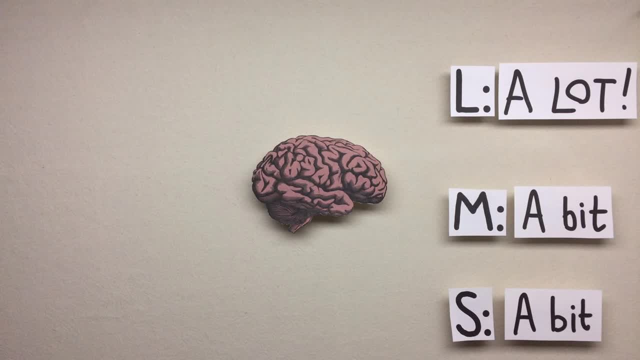 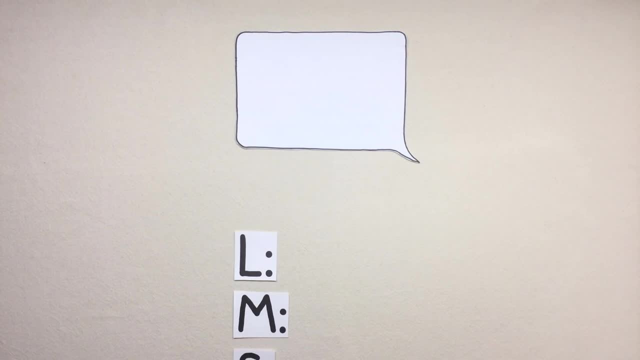 cones react a bit too. These responses make your brain give you the sensation of pink. The color sensation that we have is based entirely on the cone's reactions to the light. What this means is that if you see a red light, you're going to see a red light. 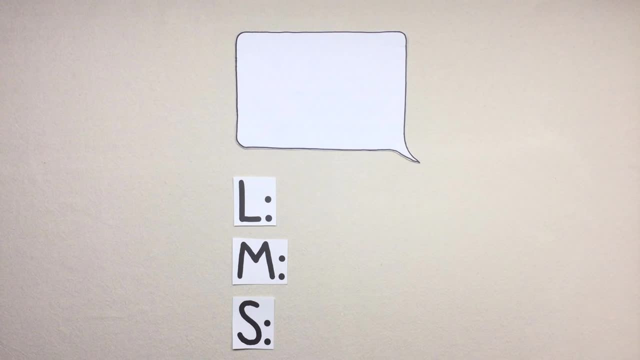 So if you see a red light, you're going to see a red light. If you see a red light, you're going to see a red light. If different combinations of light make the cones react in the same way, we'll see the same colors.